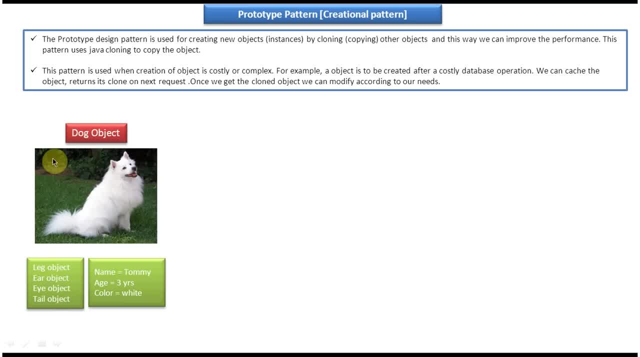 I have to use these small objects and I have to construct this dog object. So I have to create a new leg object and set the values of leg object And I have to create the ear object and set the properties of ear object And I have to create eye object. 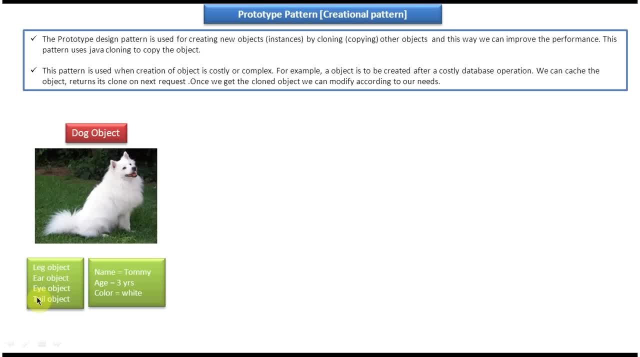 And set the properties of eye object. And I have to create tail object and set the properties of tail object. So all those things I have to do And finally I have to use this small, small object And I have to construct the dog object. 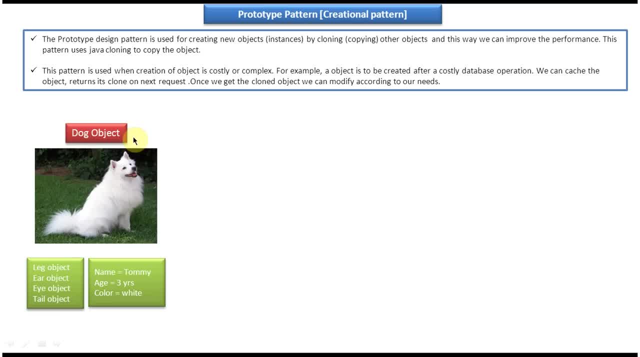 So I did this: creation of dog object. So finally, one requirement is coming. I have to create the dog object, But the color should be black And the color should be brown. All other properties are same. So what we will usually do is: 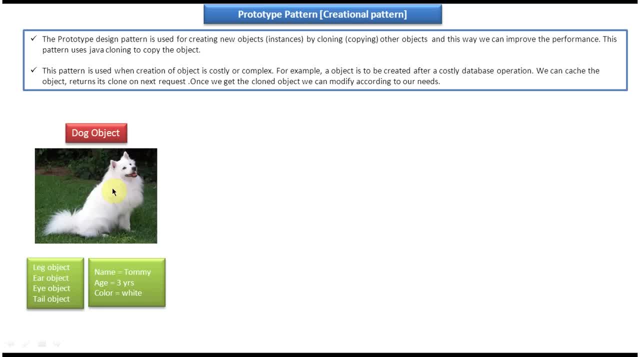 We will again use the new keyword And construct leg object, ear object, eye object, tail object, And set the name, age, color, everything And we will construct the dog object. So this is the complex operation, So we can avoid using the new operator again. 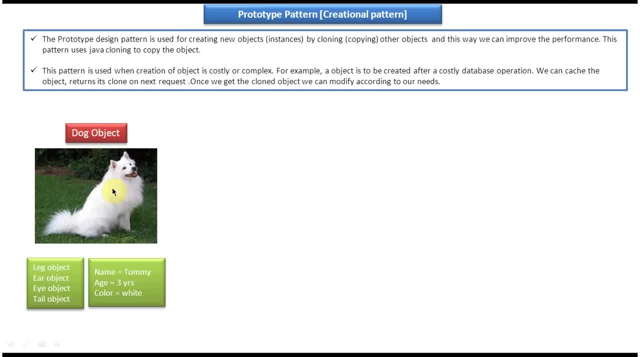 And construct the dog object again By using the prototype design button. So, as per the prototype design button, What we can do is We have to just clone the existing dog object, So we will get the cloned dog object. So whatever properties are there in this dog object, 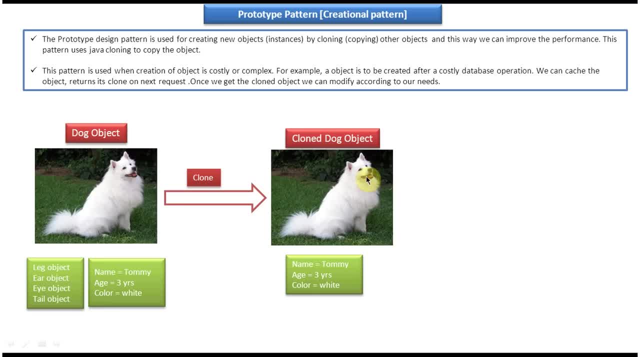 That will be available to the cloned dog object, Then my requirement is It should be a brown color dog, Right And name. we have to give some other name And age should be some other age. Okay, So what I have to do is: 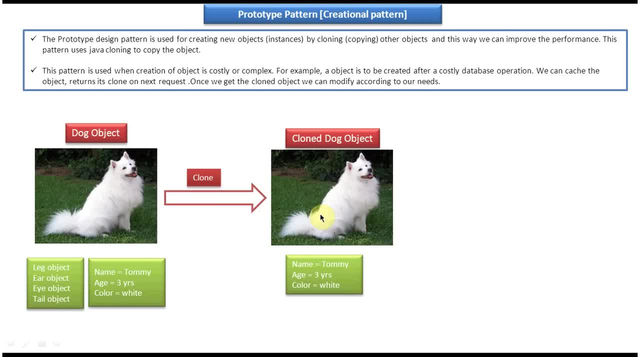 Now I got the cloned dog object Right. Then I have to just modify the This cloned dog object properties Like name Tommy to Name Jimmy, Age 3 years to age 6 years. Color white to color brown. Okay, So this way. 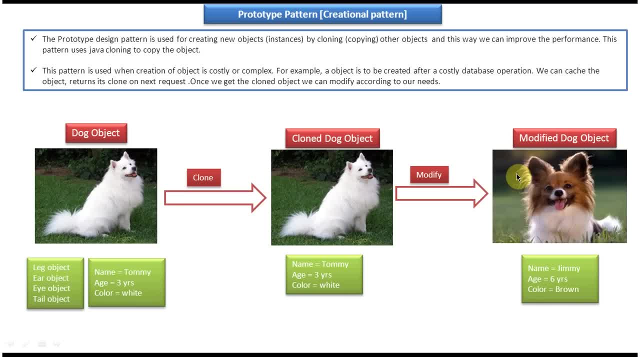 We can create the dog object very easily And we can improve the performance. Okay, So it is very simple. So we have to just first time, When the client request the dog object, We have to just construct the first dog object And put it in the hash. 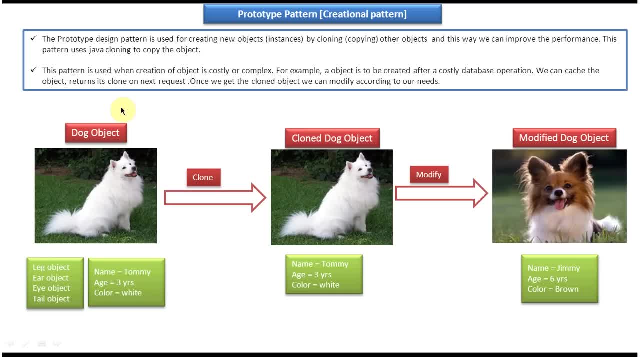 And next time when client request for the dog object, We have to get it from the hash And clone it And return copy to the client. Okay, Then once client get the copy of the dog object, Client can modify its property according to the client need. 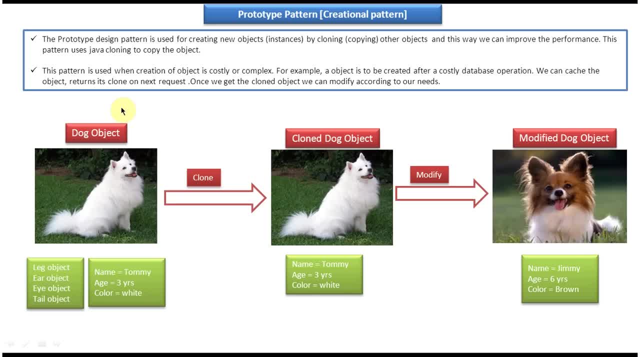 Okay, According to the requirement, He can just modify the some property And use it. So in this case, First time white color dog is created And we just cloned it. So again we got the white color dog object. Then we have just modified. 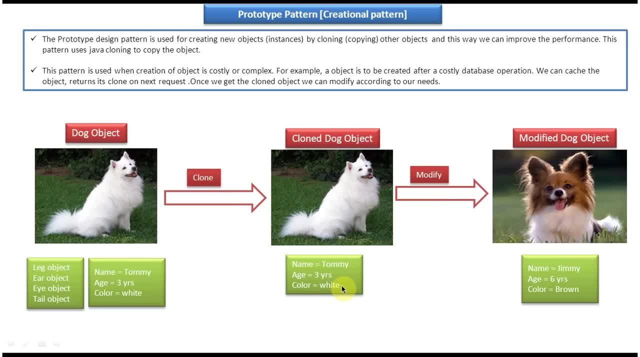 Its properties like Color: white to brown, And age 3 years to 6 years, And name: Tommy to Jimmy. So finally we got the modified dog object. So in this way we can improve the performance. Now, if I read this explanation, 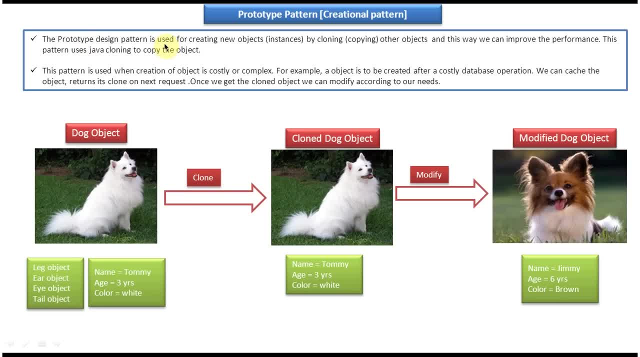 You will understand very clearly. The prototype design pattern is used for creating a new object By cloning other objects. So in this way, So in this case, This dog object is cloned And we have created other objects Right, And this way we can improve the performance. 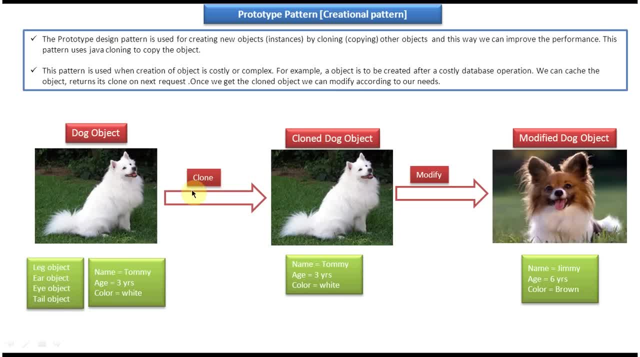 This pattern uses the Java cloning to copy the object, So the cloning. what we can do is We can use the Java cloning method And this pattern is used when creation of object is costly or complex. For example, Object is to be created after a costly database operation. 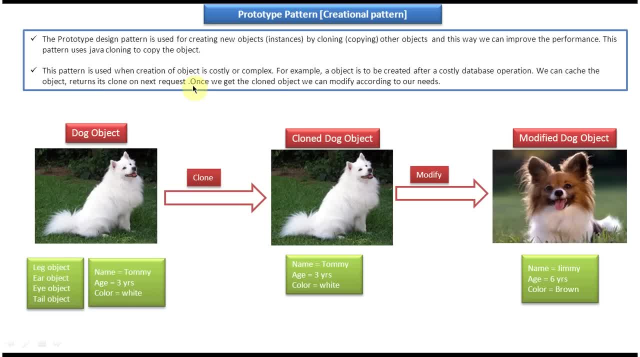 So we can hash the object, Return its clone on the next request. Once we get the cloned object, We can modify according to our needs. So here what we have done is We have cloned the object And modified according to our need. 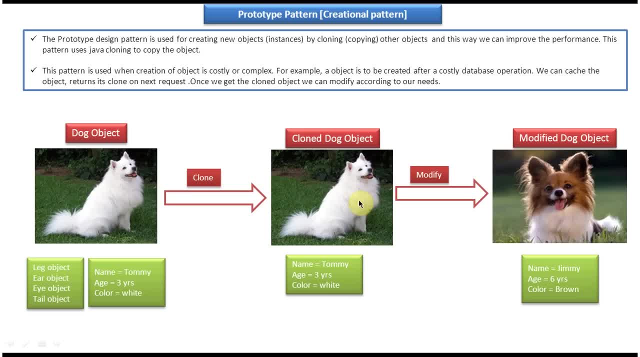 Our need is to change the color of the dog to brown Right. So we did that. So this is the best example of prototype design pattern And this is about prototype design pattern introduction, And I have created separate video for prototype design pattern class diagram.